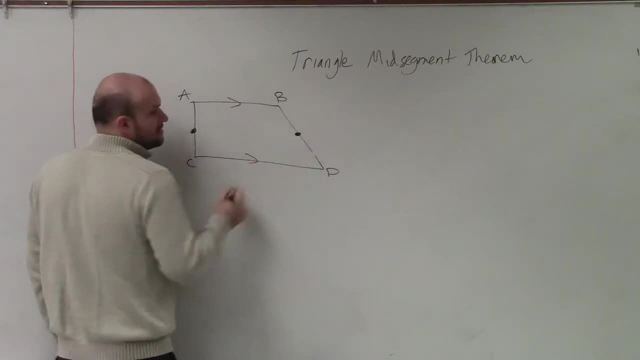 remember, oh, remember. if we can find the mid-segment of two of our legs, right, then remember the mid-segment that means they cut it in half, right? If he cuts these in half, this mid-segment is parallel to the other bases, correct, right? And then also we can find this: 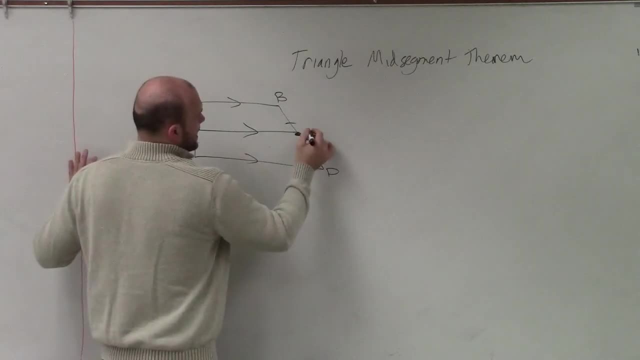 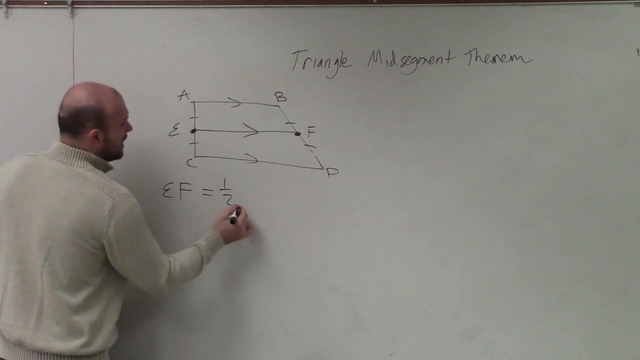 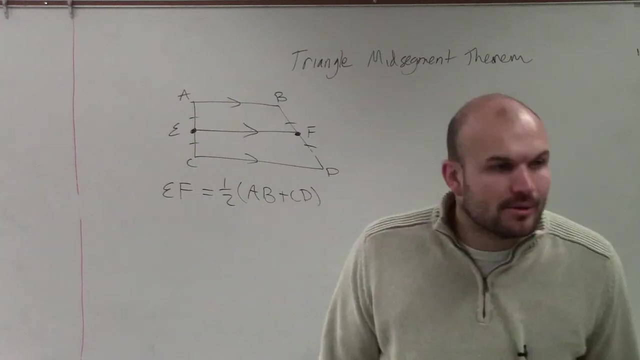 length this link. let's call this Eric and Frank. what we could say is: Eric and Frank is equal to 1: half the sum of ab plus cd. You have to know that formula for the rest of this year. That's going to come up over and over again on your test. 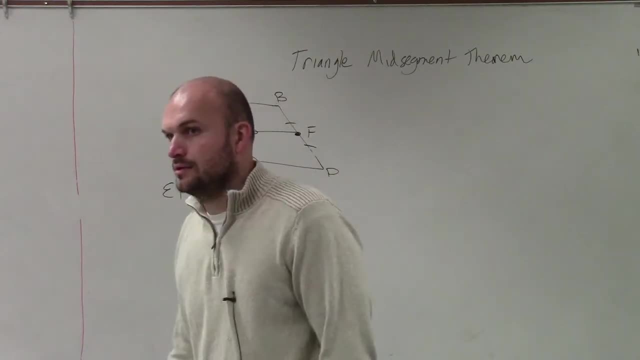 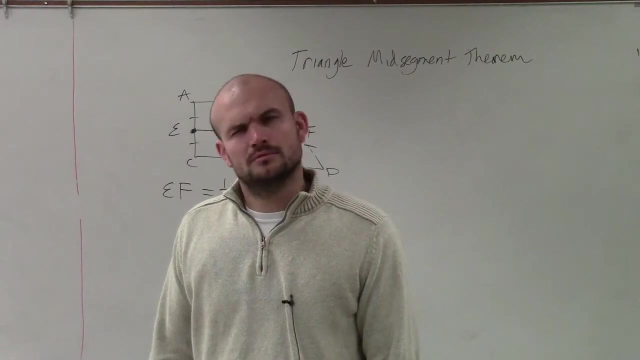 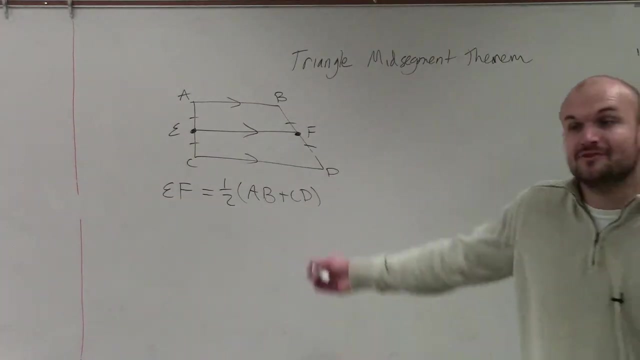 OK, I'm not sure that you were at the same time, Is that it? How does that look? So, anyways, so we have to know that formula. So if you forgot that formula, and you know it, because it's on that test that we have our last test- 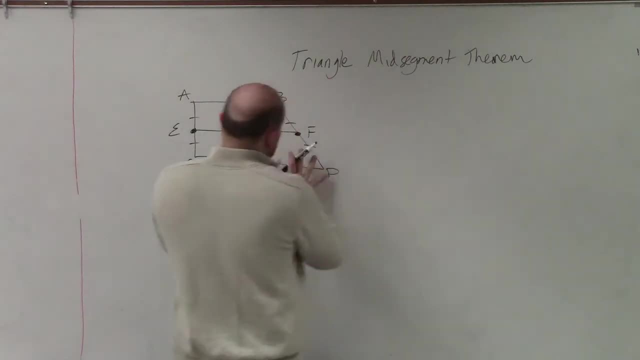 the mid-segment formula, so you want to make sure you know that. So obviously we're not talking about trapezoid, though I just wanted to review that with you Now. we're talking about the triangle mid-segment theorem. 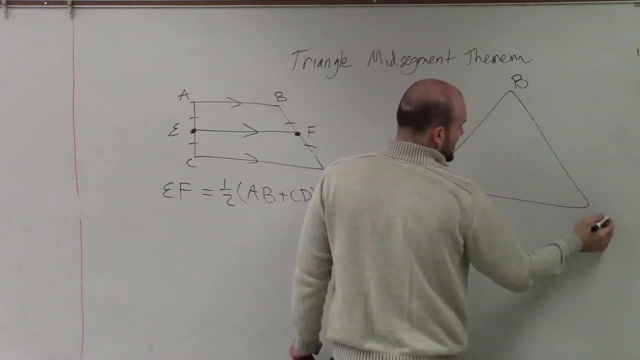 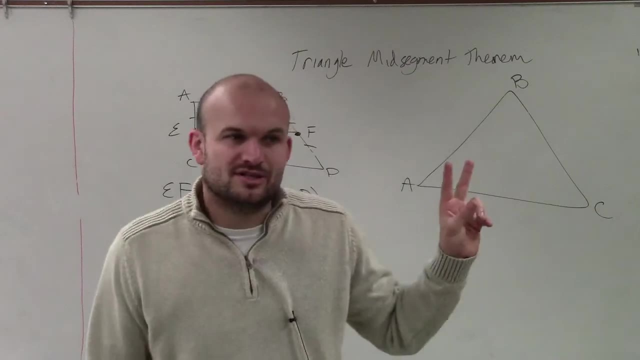 And let's just go back to Albert, Berta and Cici. OK, You have a triangle that looks like that: If we find the two mid-segments of two of our sides, let's do ab and bc. They're the mid-segments. 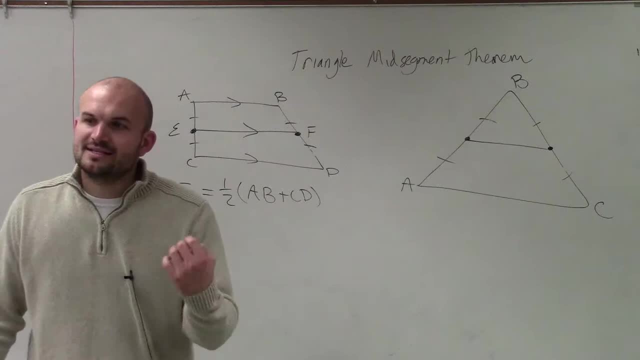 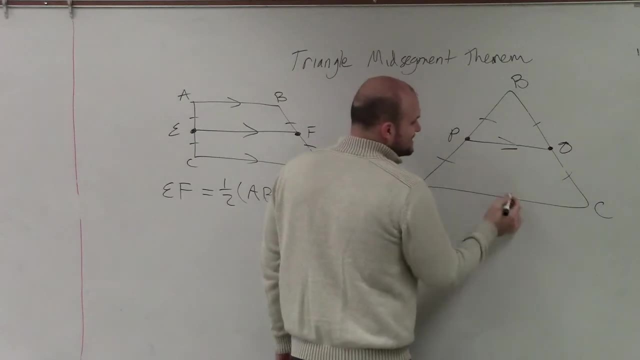 That means they cut them in half, right. What that tells us about the triangle is now, let's say: this is p and q. that says that this is now parallel to our other line. This is our other third side. all right, 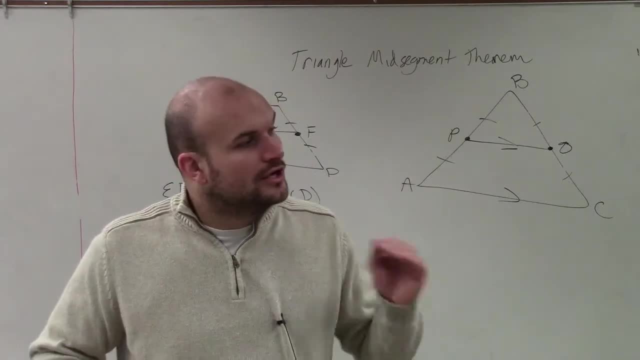 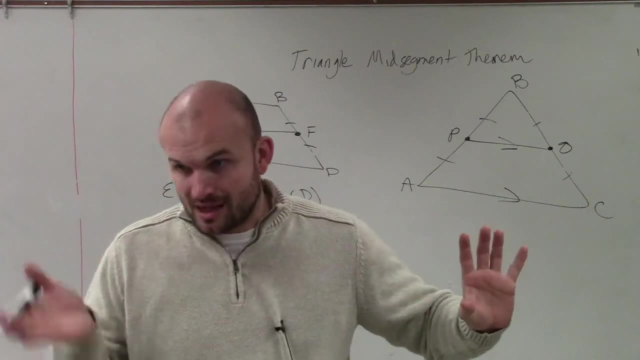 So when you have a mid-segment, if you have a mid-segment and a triangle, you now have proven that you have parallel lines, which is good because parallel lines are very important in this class, right, Because we like parallel lines and a transversal that.